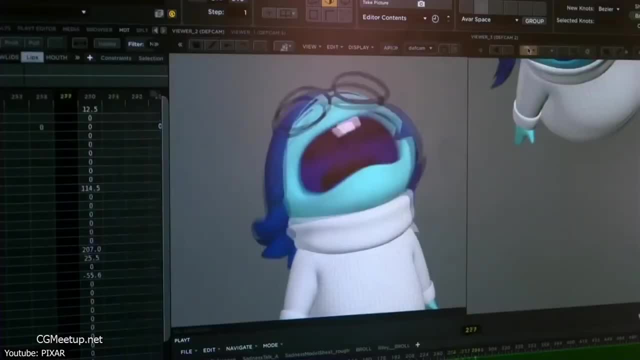 the world of 3D animation, where math is essentially the backbone of absolute science. Let's start simple, without entering the world of 3D animation, where math is essentially the backbone of absolute science. Let's start simple, without entering the world of 3D animation, where math is essentially the backbone of absolute 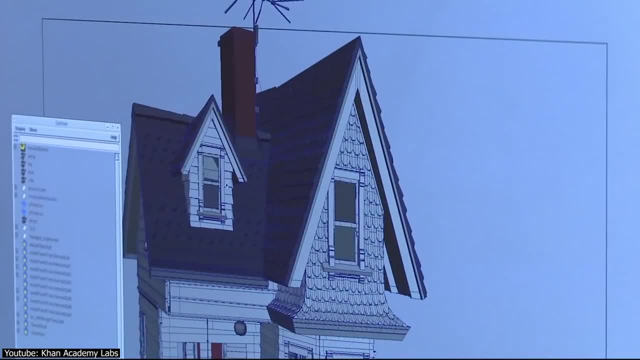 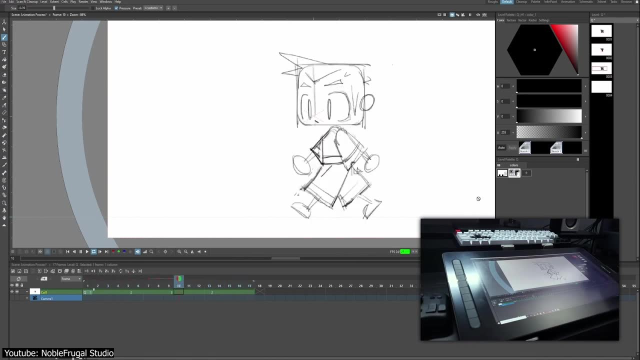 everything, since computers rendering 3D objects, sometimes in real time, are involved In 2D animation, it's important to figure out a few basic things before starting the actual animation process. In the animation pipeline, we often record voice lines and music before the animation. 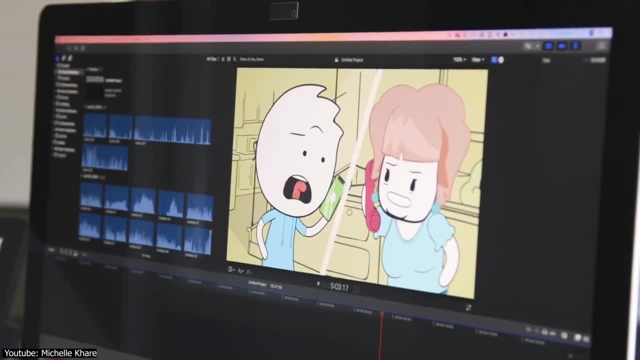 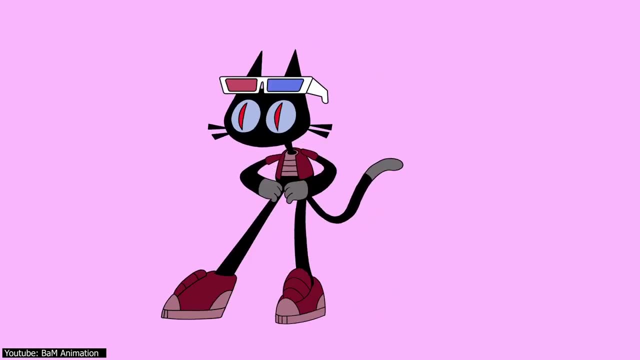 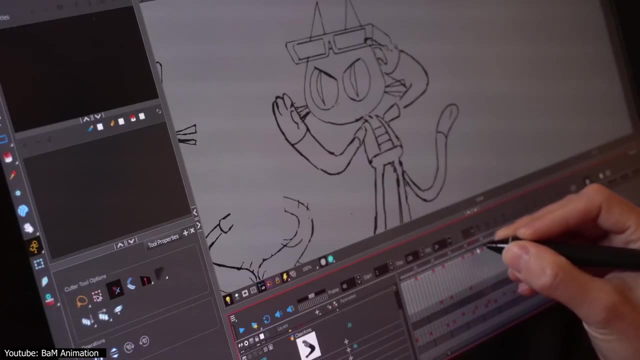 proper begins. so animators have to match the timing of certain keyframes or actions to the words of the actors or the tempo of the music. The latter elements have a very specific timing. to create TV-quality animation with 24 frames per second, the animators have to divide every action. 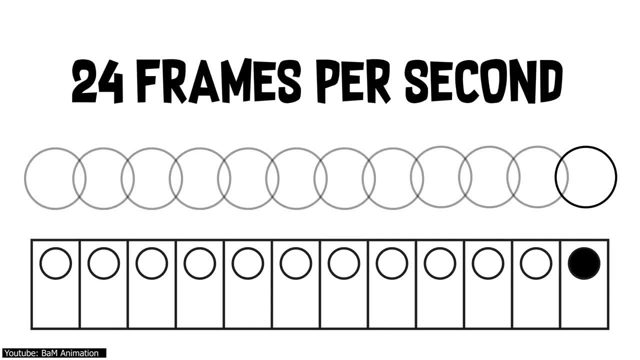 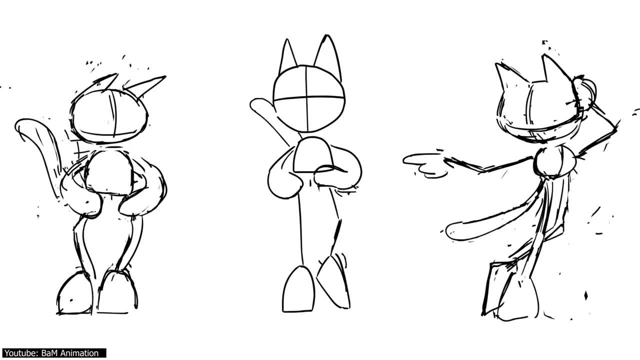 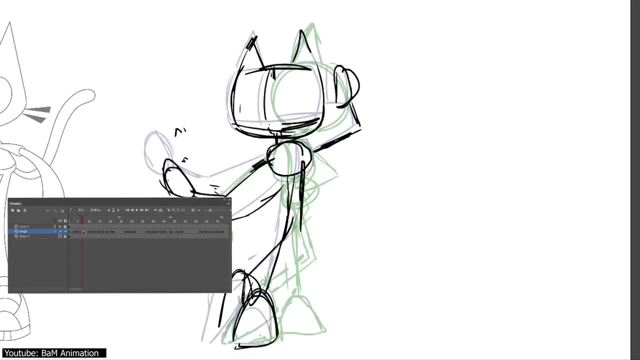 into 24 fractions of a second, But not all keyframes are placed at one-second intervals. For example, in an action scene that is to the beat of faster tempo music, we can decide to have the movements following the beat of the music, which could hit multiple times within. 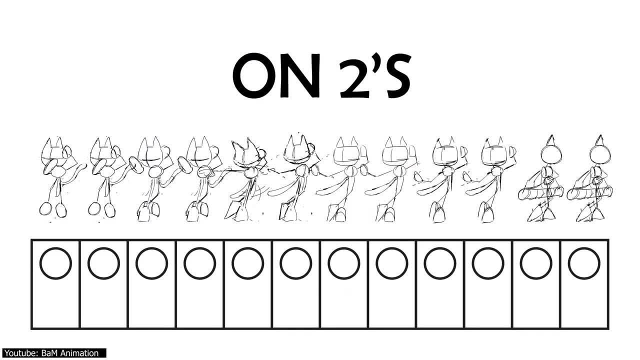 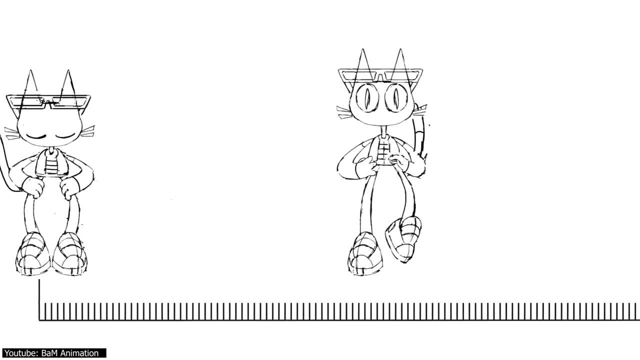 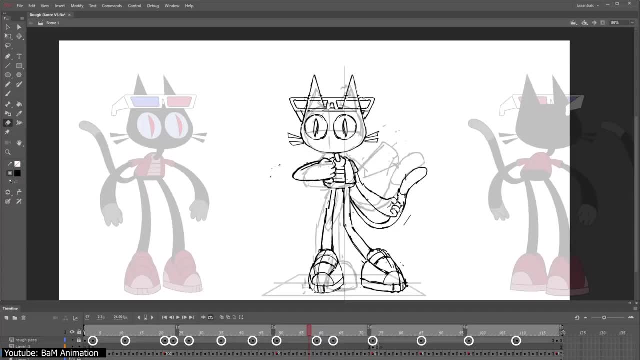 one second. For the sake of example, let's say the beat hits twice every second. That leaves us with 12 frames for every action, and then we could end up with irregular timings to match the beat, like every second and a half. Point is: you need a plan of attack, and that plan is not. 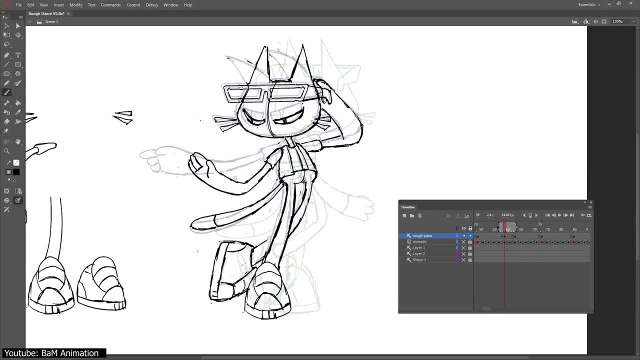 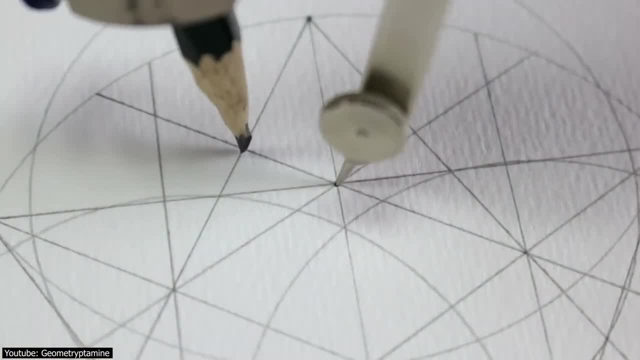 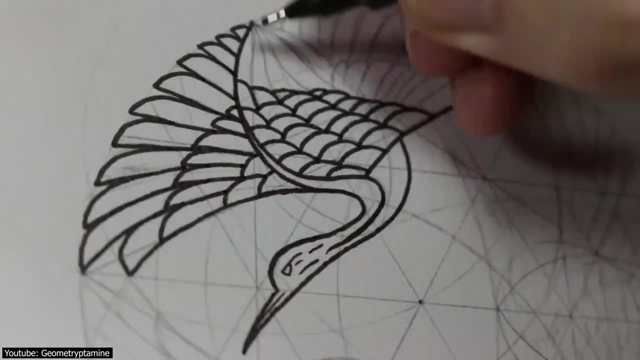 going to figure itself out. you have to solve it for yourself. For this second point, we'll talk about shapes. Oh my god, shapes, They're all fun and games. until they're not, We can agree that geometry makes the basis of all art. I'm sure that you have seen, at least 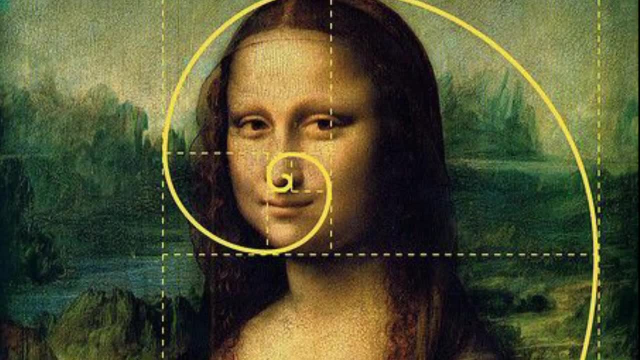 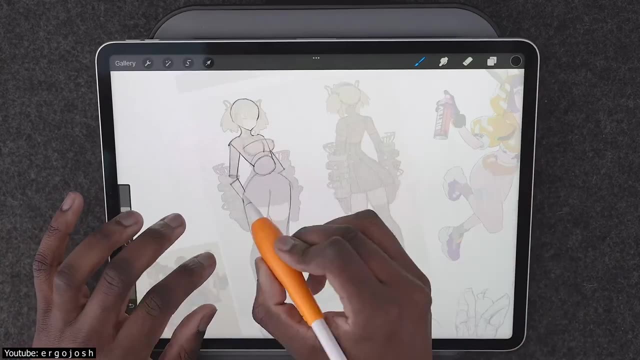 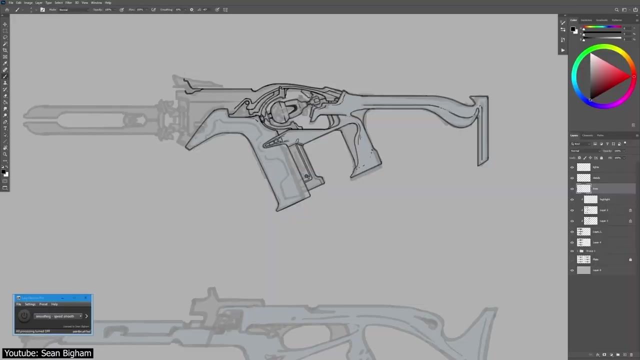 least a few paintings in your lifetime referencing the golden ratio. And that's only scratching the surface, as geometry and numbers are the basis of perspective, simplifying anatomy, the architecture of buildings, designing props, weapons and vehicles, among other things I think we made. 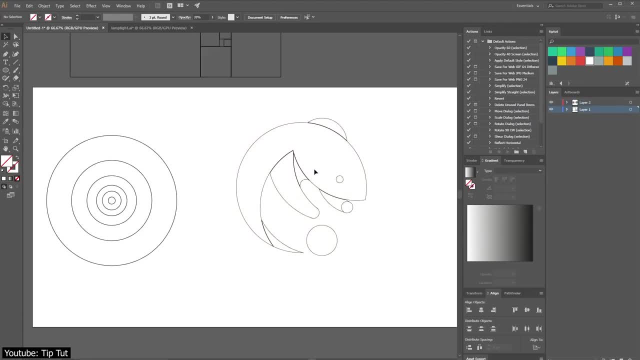 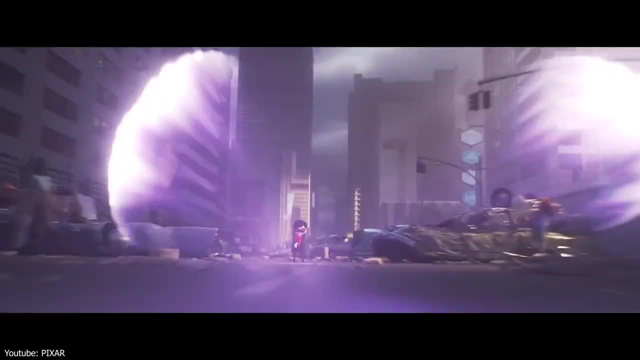 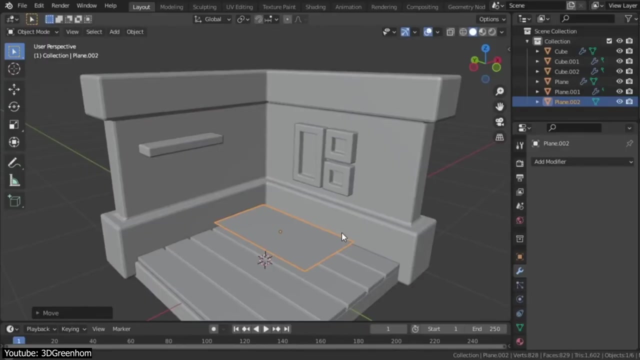 our point here. Shapes are absolutely essential when working on any art project, and geometry is essential to building said shapes. 3D animation takes this to a whole new extreme. Computers don't know what things look like, so it's up to us, the people, to try to have these computers. 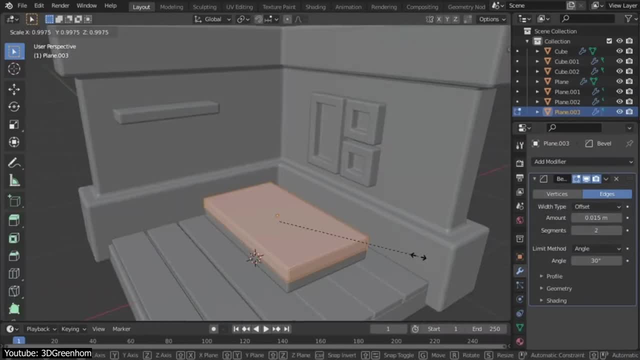 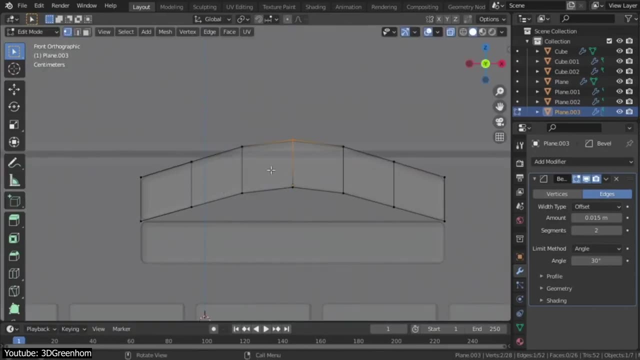 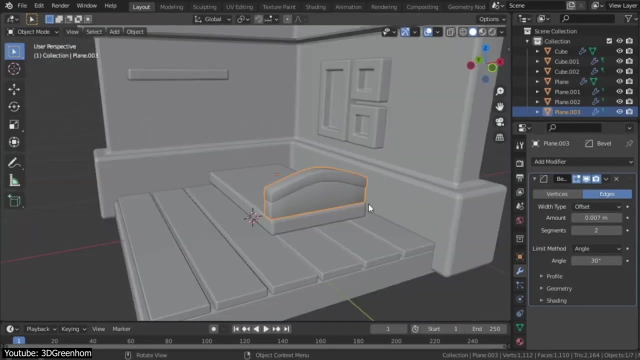 understand objects in a manner that is enough to represent them. That is done through giving them coordinates to points in a 3D space. By connecting these points we can make lines, and by having lines intersect with each other we can represent planes. And by overlapping every 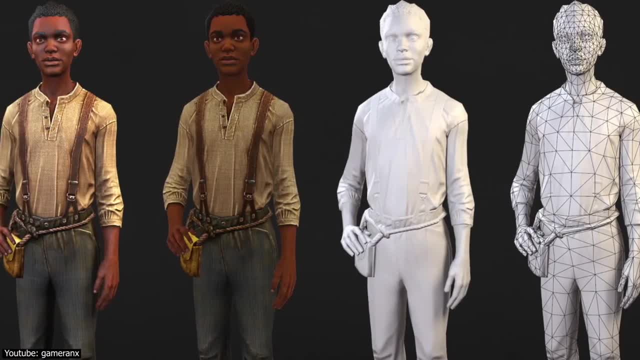 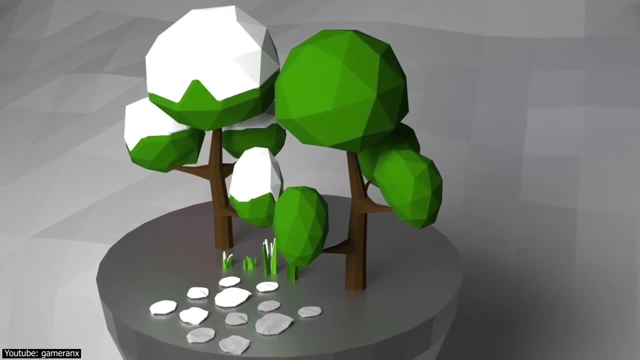 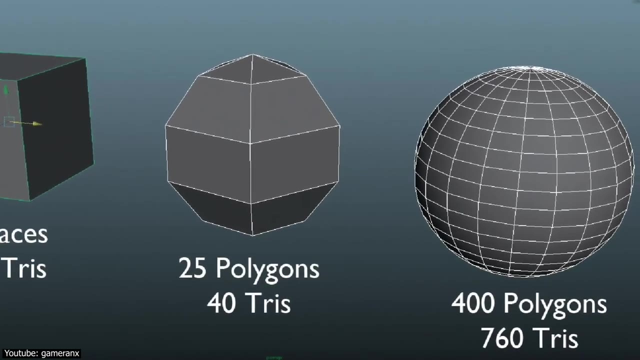 thing. together, we can form surfaces of polygons. God, we got there. Polygons are the backbone of 3D modeling. Everything is made out of polygons, and the sheer number of polygons available is what determines how smooth an object looks. This is how we actually went from triangular 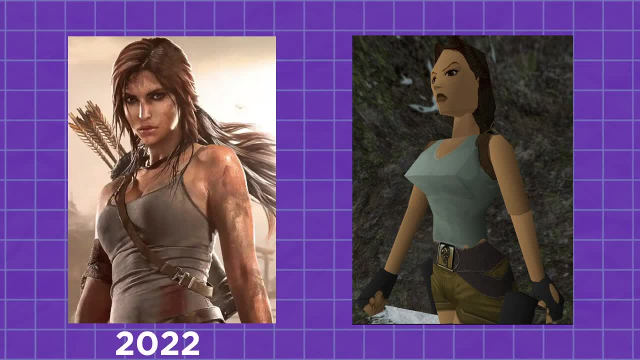 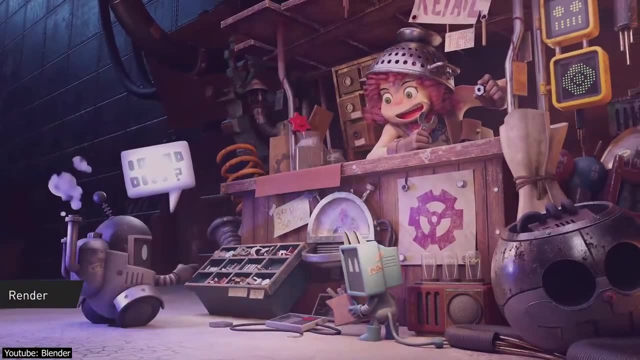 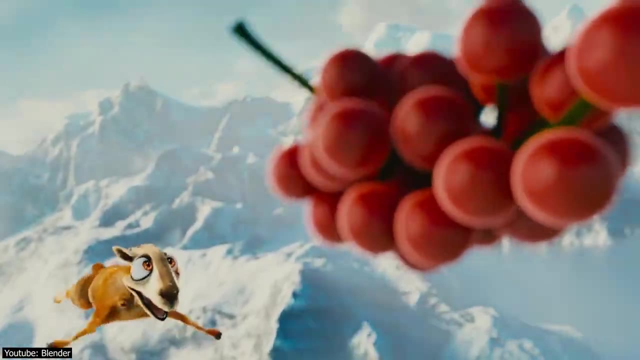 Lara Croft to regular-looking Lara Croft. The difference between them is the result of computing power being able to render a larger number of polygons at any given time. Current computers can render more polygons than their ancestors, so our current models tend to look cleaner or more realistic. The artists over at Pixar use this idea, while 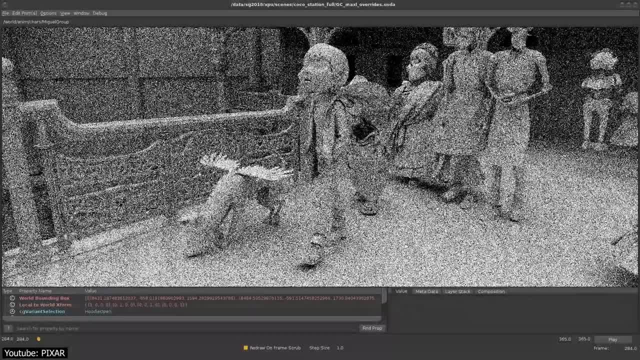 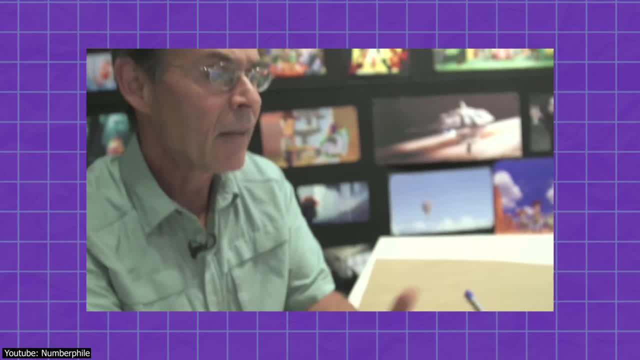 rendering their 3D models to have them look as smooth and natural as their technology can muster. There's this incredible video by Numberphil that goes into more detail about the numbers behind 3D models And, speaking of rendering, there's a whole equation for 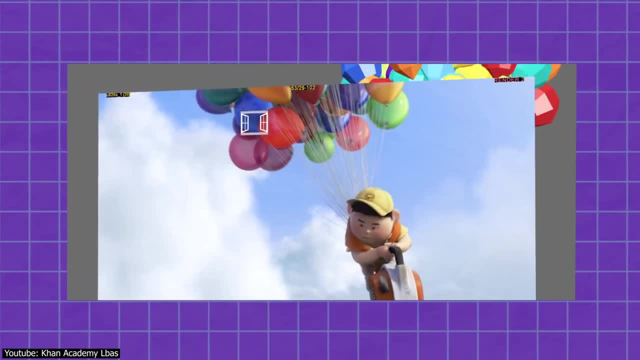 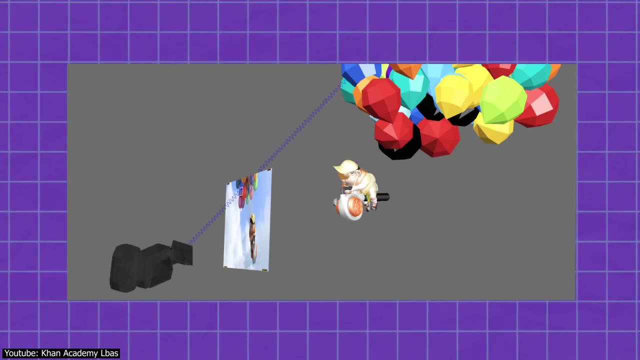 the rendering process that takes into account light and light. We won't get into that here because it's not something that can be explained in a short format video. Just bear in mind that it can get very complicated very fast. I mean look. 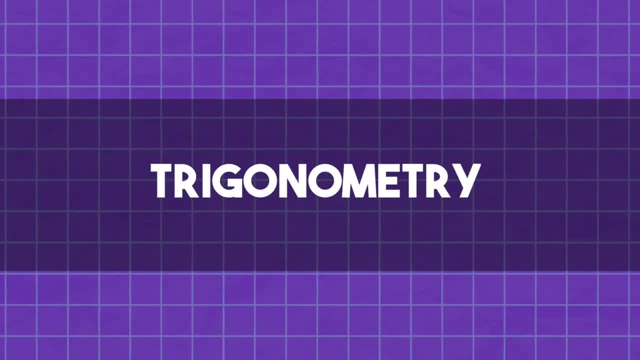 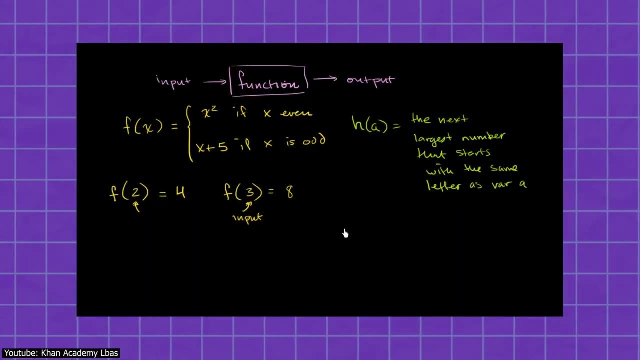 at this In the topic of equations. do you all remember functions, How they can be represented by a graph or an equation? And then we had that whole thing about right triangles and their sinuses and cosines and the relation between them and all that fun stuff. 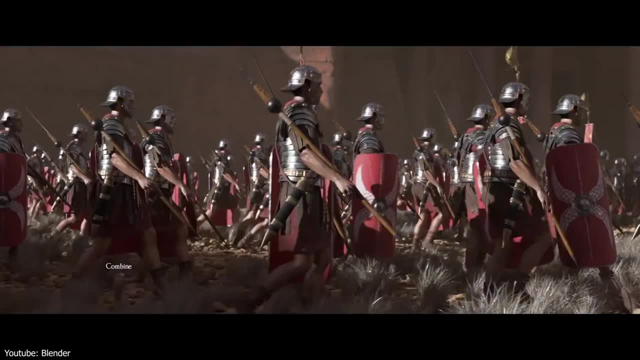 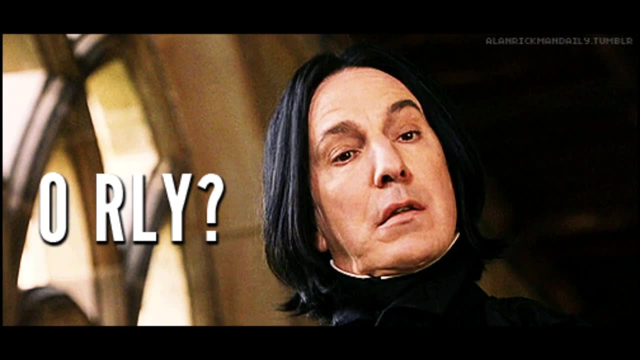 I really can't imagine how those can ever be useful in 3D animation, Am I right? It's essentially how all animation is done: Trigonometry, Really. now, As I hear your sighs across the vastness of the ocean, let me explain. 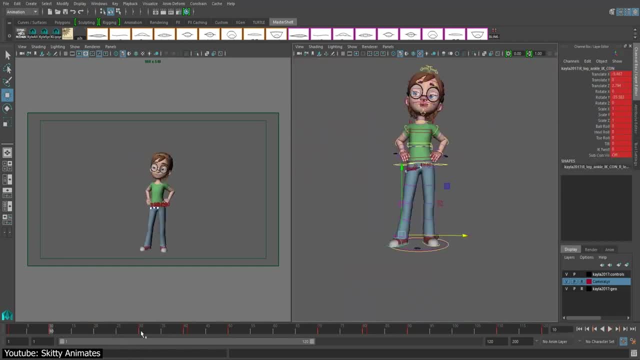 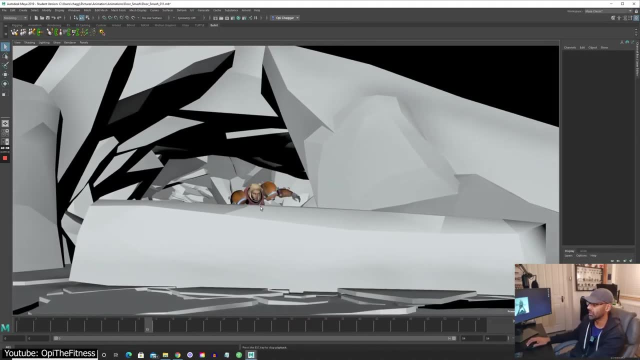 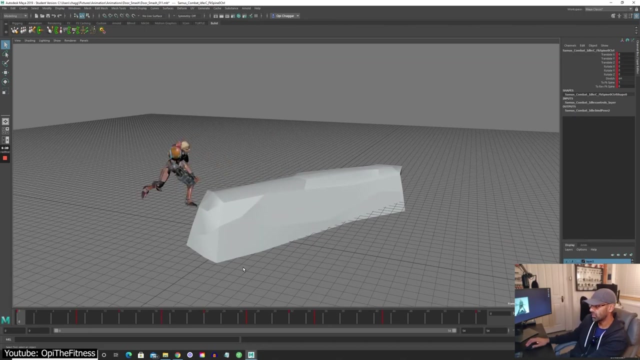 In computer animation we move digital 3D models in a process called posing, where poses are recorded by the computer in the form of coordinates. The computer then tries to fill the gaps between these poses by creating in-betweens. These in-betweens represent how the computer thinks an object will move from pose A to. 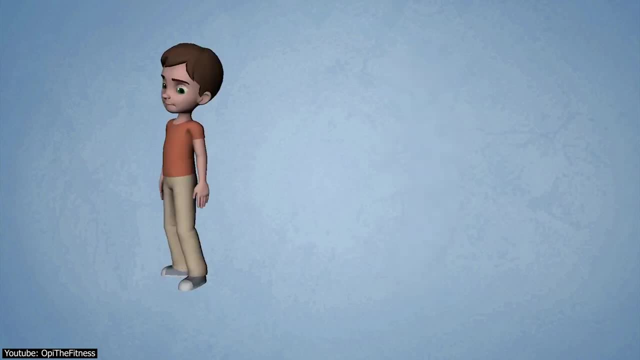 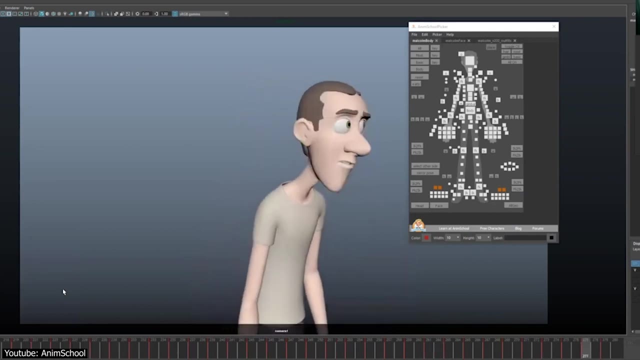 pose B. These in-betweens can be described using a mathematical function called a spline that can later be manipulated to give the animation a more natural movement and flow. The cosinuses and sinus graphs are splines that represent the movement of a singular. 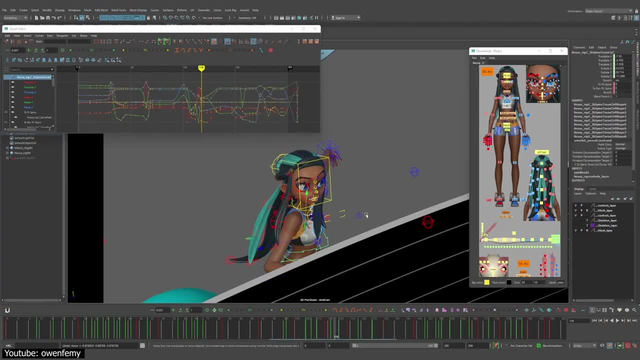 point through the circumference of a circle. Other splines are a representation of other types of movement. All that being said, computers will have a lot of fun with these in-betweens. So let's get started. We'll have the tendency to make a linear interpolation of motions, and we'll always 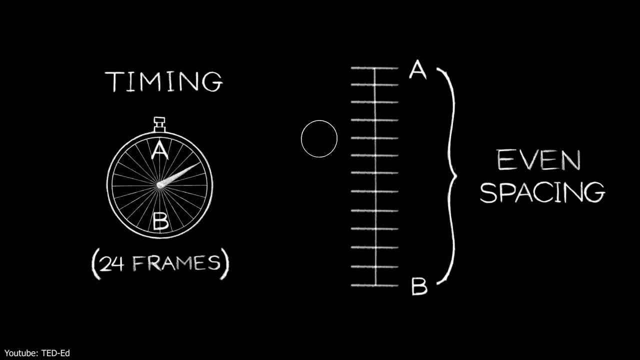 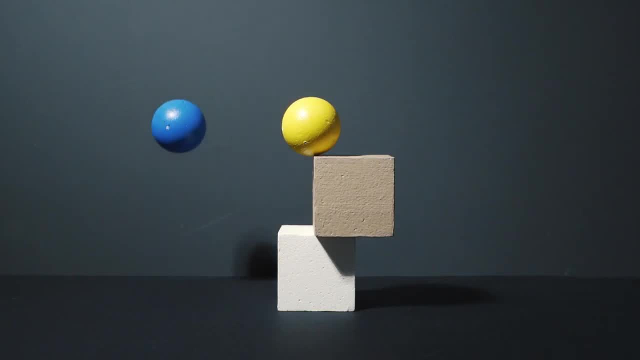 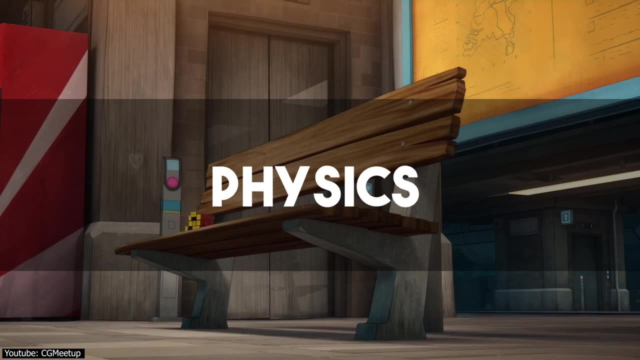 have the objects move at a constant speed. This is where manual intervention is required to make the timing of said movements more accurate to how it would be in real life and more realistic when taking into account the laws of physics. Speaking of the devil, it's Matt's favorite love child physics. 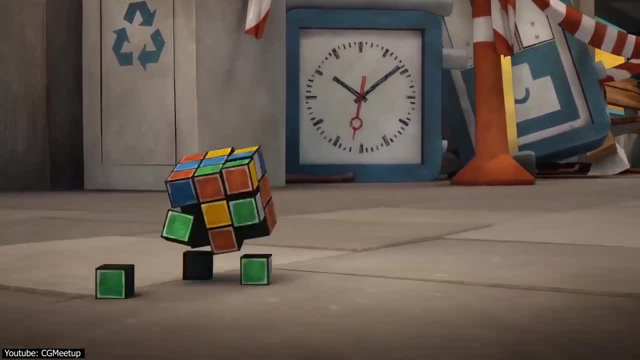 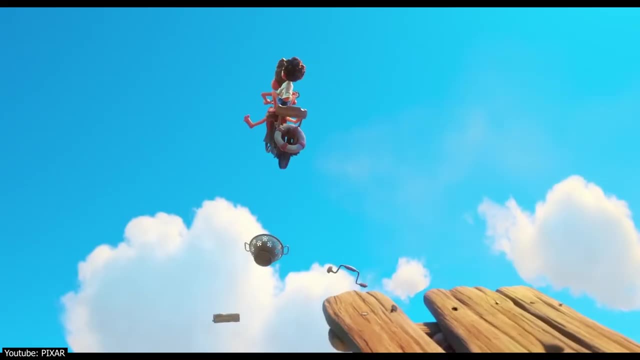 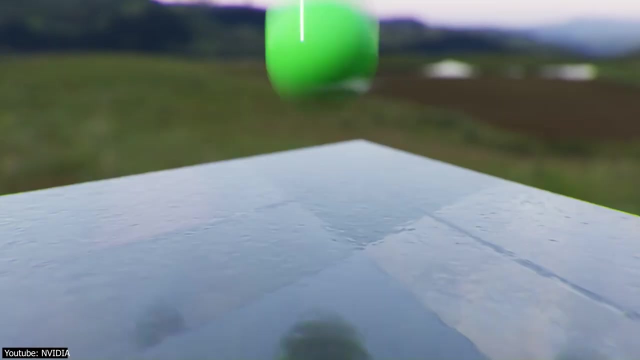 Animation is all about creating the illusion of movement, and movement is ruled by the laws of physics. A fundamental understanding of these laws is essential to creating natural, flowing and believable animation. Either that, or you know people creating entire physics engines that will accurately simulate 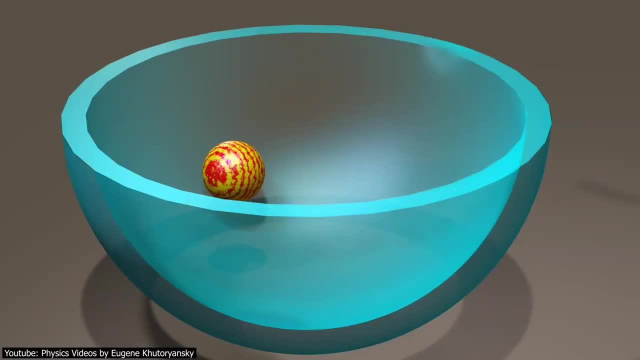 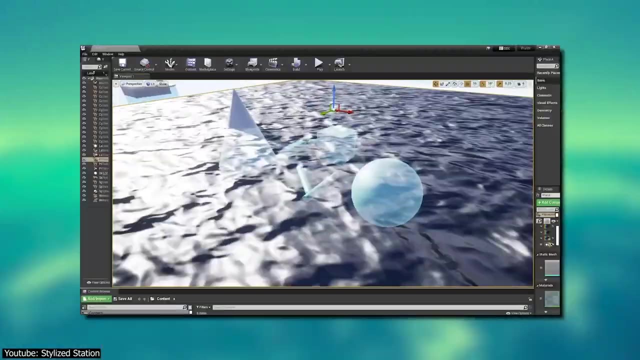 how objects will behave in real life without needing to actually manually animate them, Like in the game of Sea of Thieves. the waves are procedurally generated using vertex displacement, following the Gerstner formula, which simulates the movement of ocean water using an ocean. 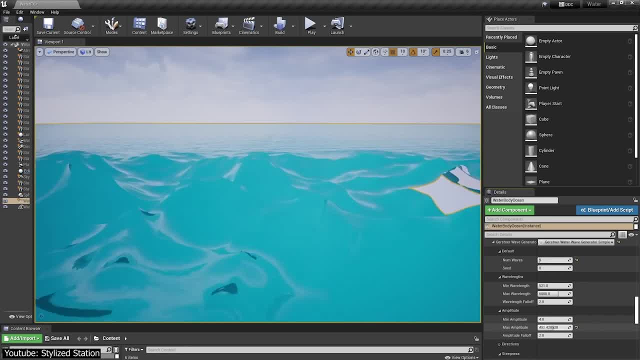 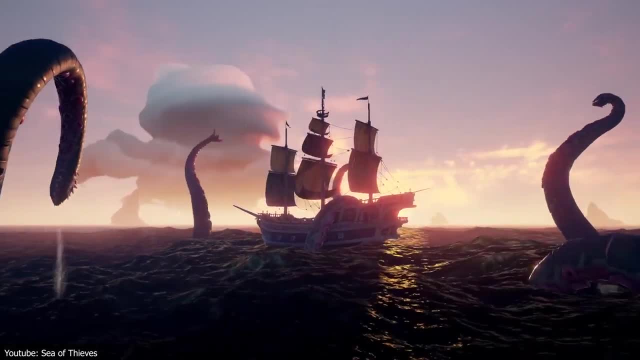 overlap of sinus waves with different intervals and magnitudes. With those, you can create a surface that ripples exactly like water. Okay, those were a lot of big words, I get it, But the point is the computer can use complex equations that are used to describe phenomena. 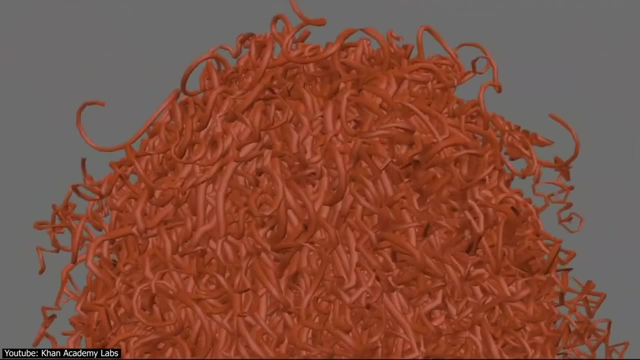 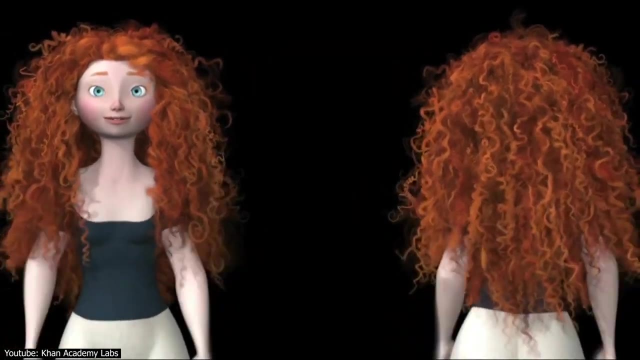 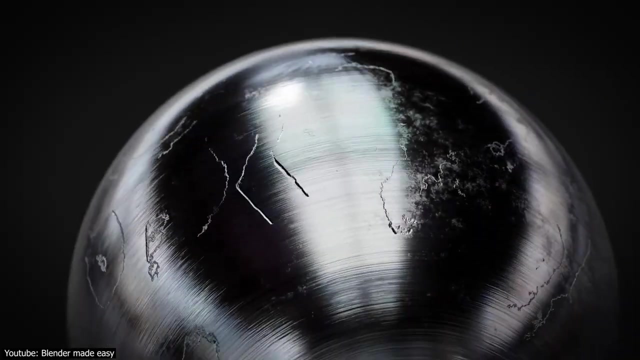 in real-life physics to recreate a simulation of them that is more accurate digitally. And that's just movement. The same principle can be applied to shading and materials and their behavior in each other's presence. We are at a point where material-based rendering is the norm, where 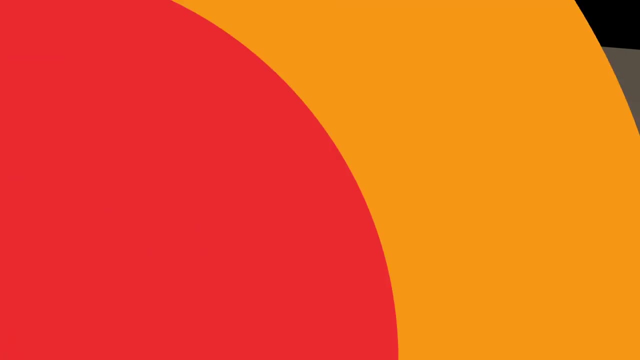 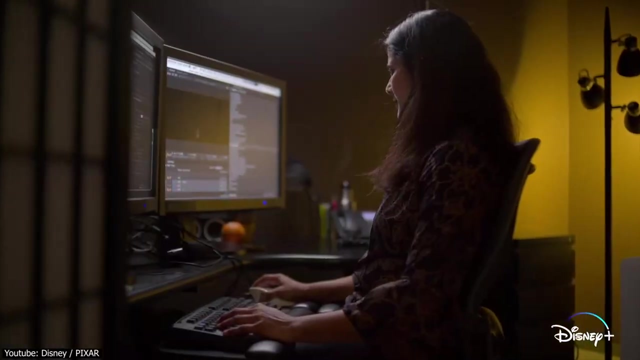 materials behave like they are supposed to do in real life. Well, there you go. We hope we haven't burst your bubble too much with this subject, as math is absolutely integral to anything computer related, but also is very relevant in traditional animation, especially during the planning phase.